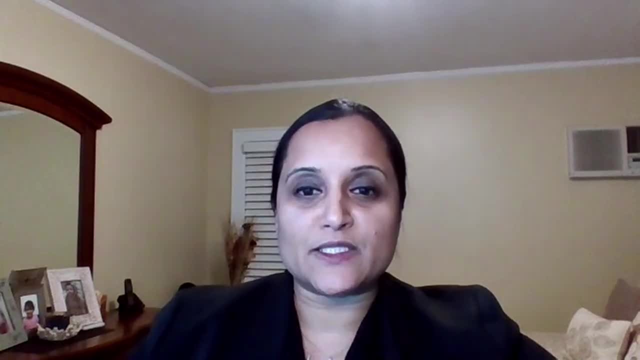 for social studies, which includes being a board member and a publisher liaison for the Long Island Council for Social Studies, co-chairing the Cultural Education Committee for the New York State Council for Social Studies, and I'm an active member of the Advisory Council for Rho Kappa National Social Studies. 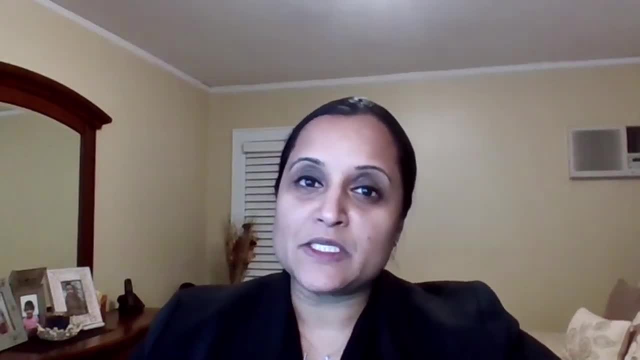 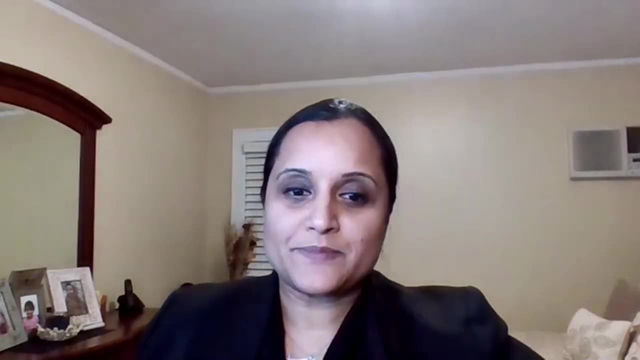 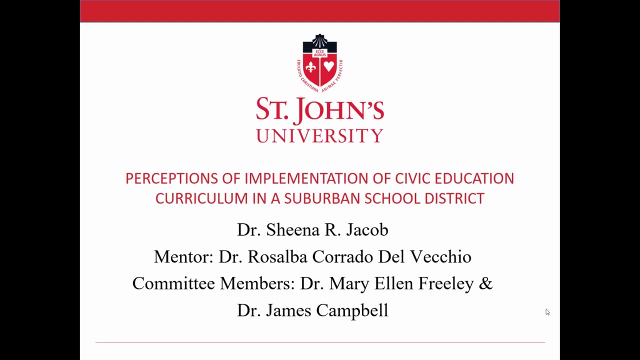 I'm excited to be here with you today to discuss my dissertation. Thank you for this opportunity. My research focuses on the perception of implementation of civic education curriculum in a suburban school district. Before I continue at this time, I would like to acknowledge my mentor. 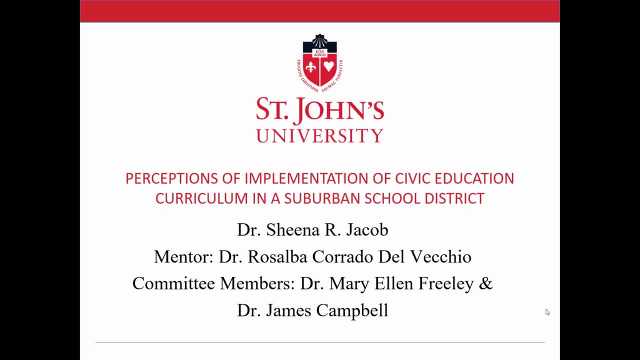 Dr Rosalba Corrado del Valle, who worked very close with me, to me, to with me, and with her guidance and knowledge I truly evolved from a student of research to an academic researcher. and my committee members, Dr Mary Ellen Frehley and Dr James 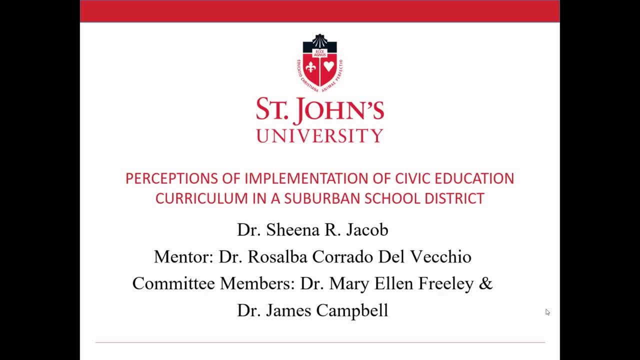 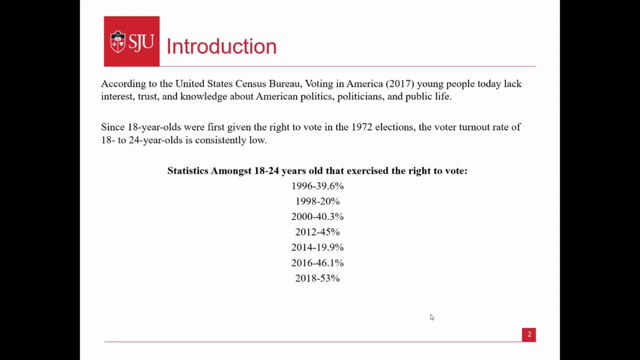 Campbell, who supported and provided me with an incredible insight for a successful dissertation and research In this research. civic education involves curriculum elements such as courses, resources, programs that include guest speakers, assemblies, projects, portfolios, and urges students to understand, engage and participate in the curriculum. 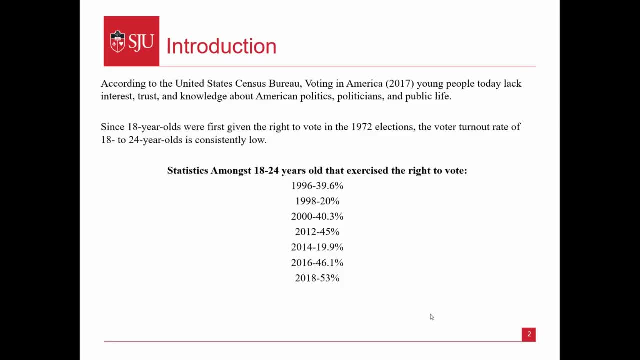 There are many different ways to engage in civic activities at the local, state and national level. According to the United States Census Bureau of Voting, in America young people today lack the interest, trust and knowledge about American politics, politicians and public life. 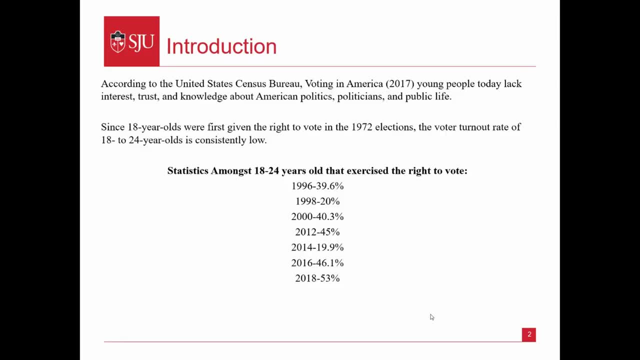 Since 18-years-olds were first given the right to vote in the 1972 elections, the voter turnout rate of 18- to 24-year-olds is consistently low. The lack of participation in voting could indicate the lack of emphasis of civic participation. 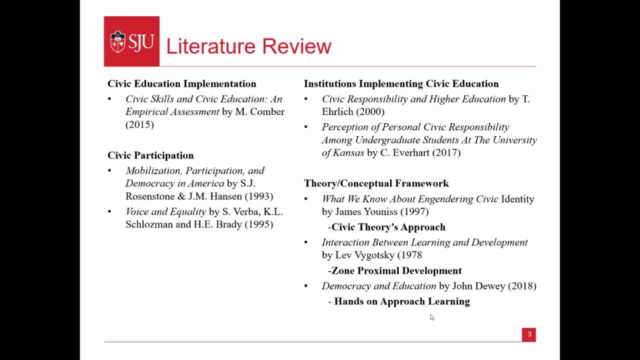 amongst its use To support this study. research that was used in this study in the literature review section includes and supports civic education implementation, civic participation and research that can be found at the higher education level that supports institutions implementing civic education- Two articles that supported the institutions implementing civic. 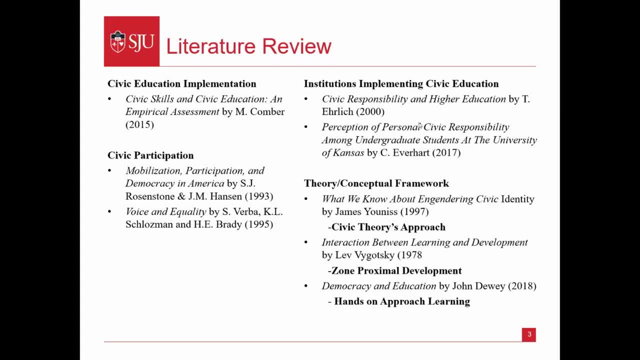 education include Civic Responsibility at the Higher Education by T Elric and the Perceptions of Personal Civic Responsibility Amongst Undergrad Students at the University of Kansas by C Everhart in 2017.. To take a closer look at the Civic Responsibility in Higher Education by T Elric, the 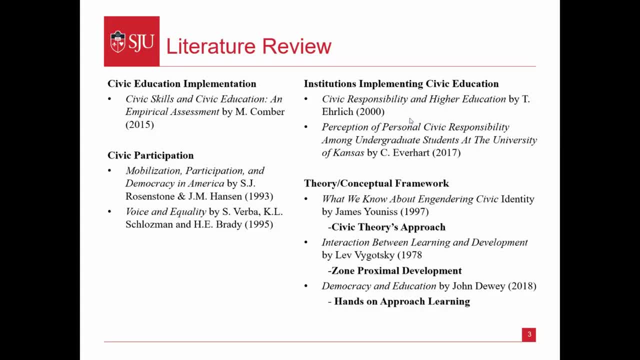 research supports essays by professors in higher education, and the center focuses on John Dewey's mandate that American democracy requires civic engagement to realize the potential that citizens in communitiesbedu of. that is the key to engagement In the Perceptions of Personal Civic Responsibility. among 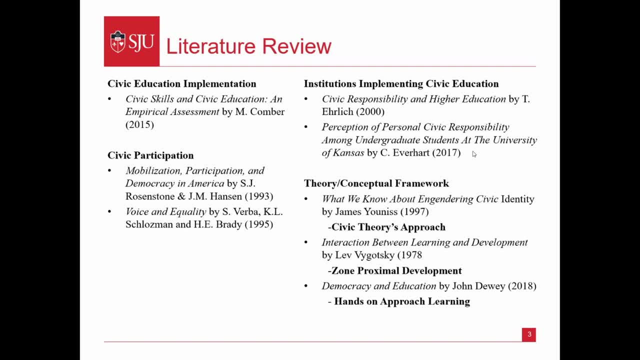 undergrad students at the University of Kansas C Everhart uses and focuses on his study. Identifies the Predictors of Students' Perceptions of Personal Civic Responsibility, civic mightiness among undergrad students at Kansas University, C Everhart uses specific data: the 2015 multi-institution 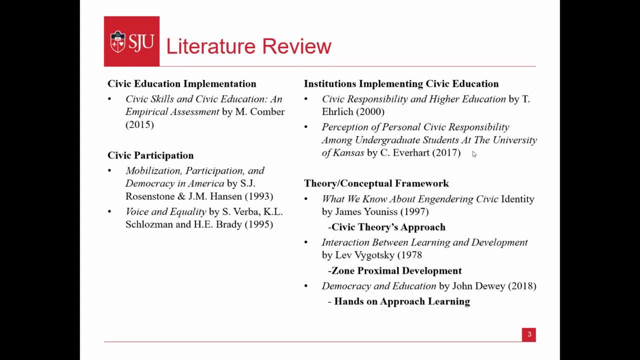 study of leadership and it correlates the relationship between Kansas University institution environment and self-reported perception of personal civic responsibility. Prior research in his study suggests the self-efficacy for civic engagement and the intentions to become civically engaged result later on civic engagement. In addition, in this qualitative study, 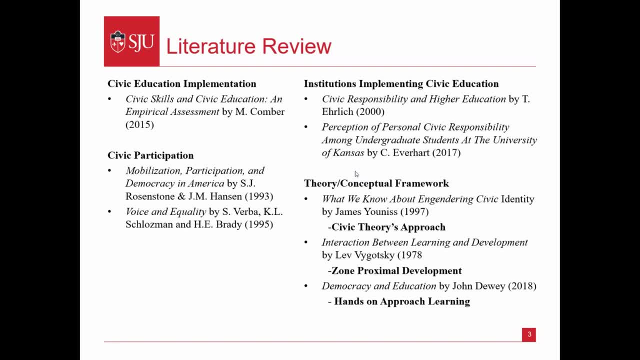 the theory conceptual framework supports the three theories: civic theories, approach zone, proximal development and hands-on approach learning. The civic theory approach can be found in What We Know About Engineering. Civic Identity by James Yunus. Interaction Between Learning and Development by Lev Vitasi supports his own proximal development. 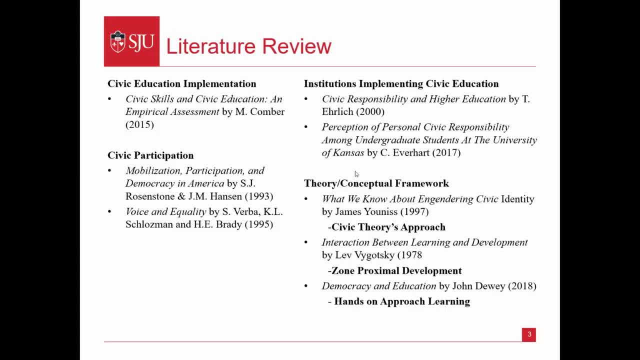 and the Democracy and Education by John Dewey on the hands-on approach learning These theories and conceptual framework. it's important to know that this is used as a guide in qualitative research, because you cannot box in a theoretical conceptual framework because qualitative you can find other frameworks as you proceed on with this study. 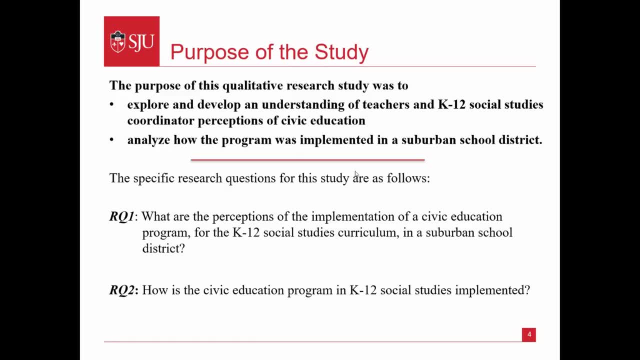 The purpose of this qualitative research study was to explore and develop an understanding of teachers and k-12 social studies: coordinated perception of civic education. The study was also to analyze how the program was implemented in the suburban school district. The specific research questions for the studies are as follows. 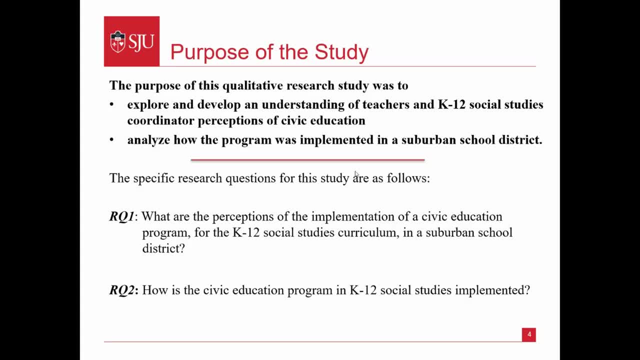 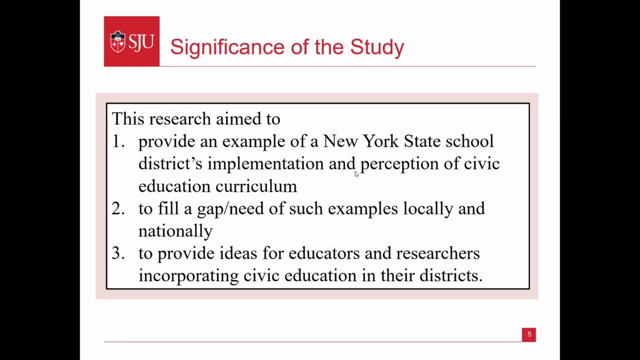 Research Question 1.. What are the perceptions of the implementation of civic education program for the k-12 social studies curriculum in the suburban school district? Research Question 2.. How is the civic education program in k-12 social studies implemented? The research aims to provide an example of New York State School District's implementation and 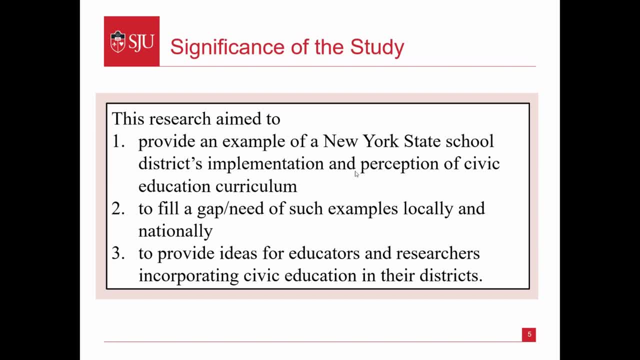 perception of the program. The study aims to provide an example of New York State School District's implementation that is appropriate for the k-12 educational curriculum. The study aims to provide an example of C war. It aims to fill vary and need of such examples. 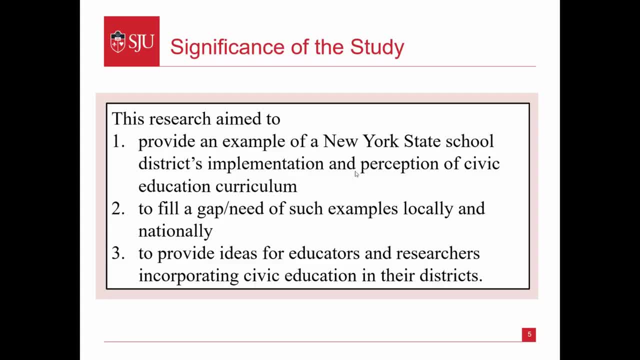 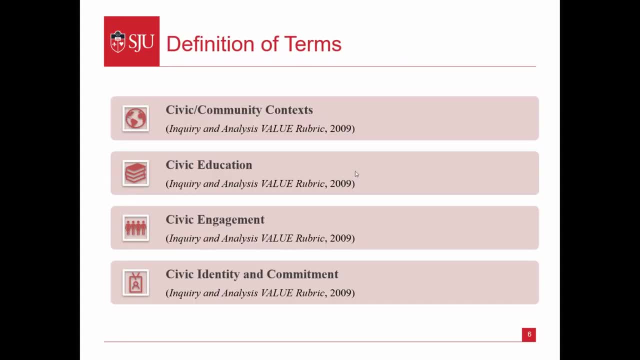 locally and nationally. The study aims to provide ideas for educators and researchers incorporating civic education in the стрicks. The definitions and terms in the study are the following: Civic community education- civic engagement- civic education. civic community engagement- civic identityれた. civic engagement- civic identity. 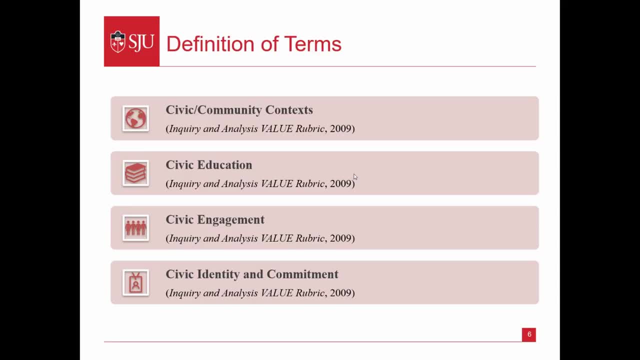 Eren mitigation civic arrangement multiple. the definitions from the Association of American Colleges and Universities, where faculty and experts representing colleges and universities across the United States examined many campus rubrics and related documents and, from each learning outcome, incorporated additional feedback from faculty members And they developed this. 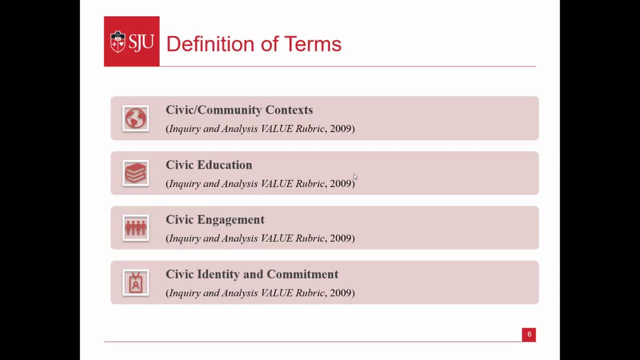 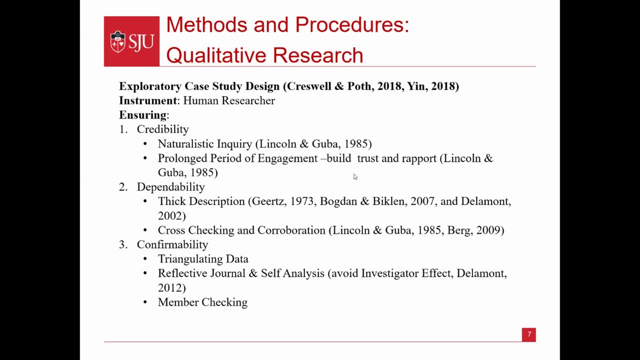 inquiry analysis value rubric, where it identifies these terms and definitions. In this qualitative research study, the research is an exploratory case study, designed The instrument is the human researcher and ensuring credibility, dependability and confirmability: Credibility, the naturalistic inquiry and a prolonged period of engagement. 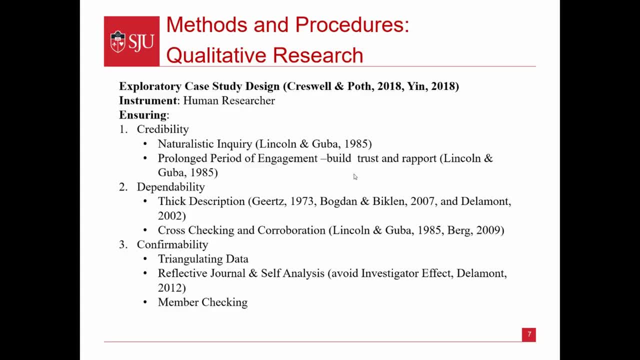 which to build trust and report took place. Also, in dependability, thick description cross-checking cooperation take place, plug during and do and place procedures of place and confirmability. the researcher myself triangulated the data reflective journal and 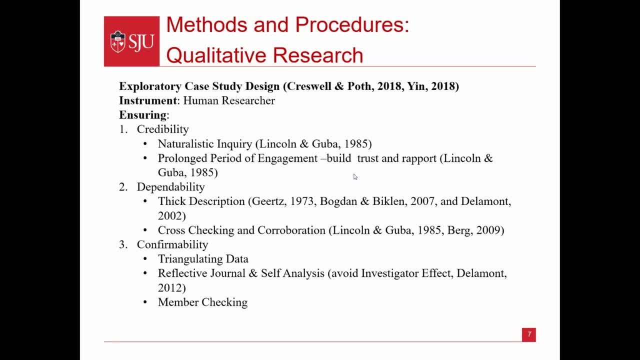 self-analysis and member checking was done. Qualitative researchers interview and observe participants to gain a deeper understanding of the participants in a way that cannot be captured by quantitative measurements of, such as surveys or other instruments. The case study methodology is best used to understand the participants' feelings, perception, understanding of the topic. 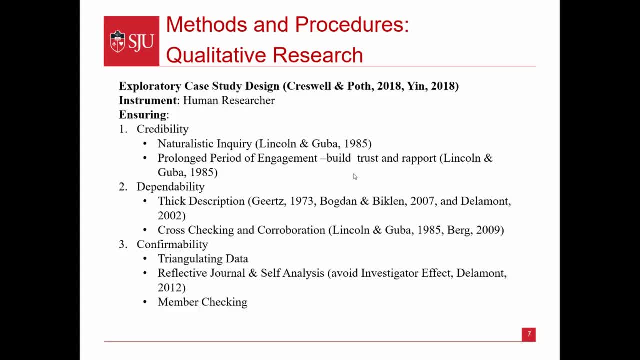 that is being researched. The case study can further be characterized as exploratory rather than explanatory. An exploratory case study, according to Berg 2001,, is typically used as an intuitive investigation that is made in the early stages of detailed research being conducted. 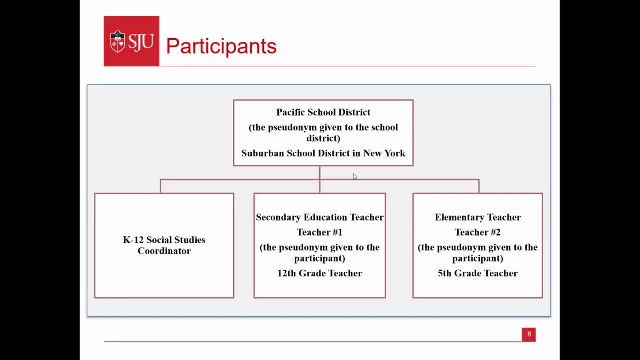 in a particular area, such as the area of interest in this study. The school district that was used in this study was called Pacific School District. That's the pseudonym given to the school district. It is located in a suburban school district in New York. It has one high school. 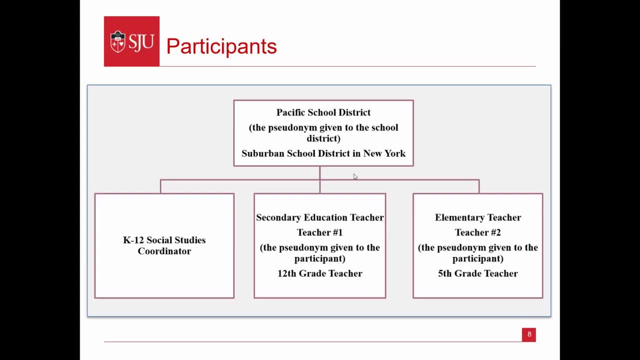 from grades 9 through 12,. one middle school- grade 6 through 8, and three elementary schools from grades K to 5.. The K to 12 social studies coordinator also participated Four years in the school district, 12 years as a teacher, Secondary education teacher, which is known as. 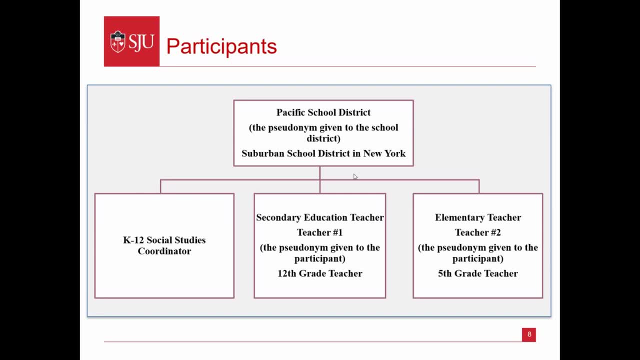 teacher number one. the pseudonym given to the participant was a 12th grade teacher who has 16 years of teaching in the district and is a Long Island Council for Social Studies and New York State Council for Social Studies member. An elementary teacher. teacher number two. 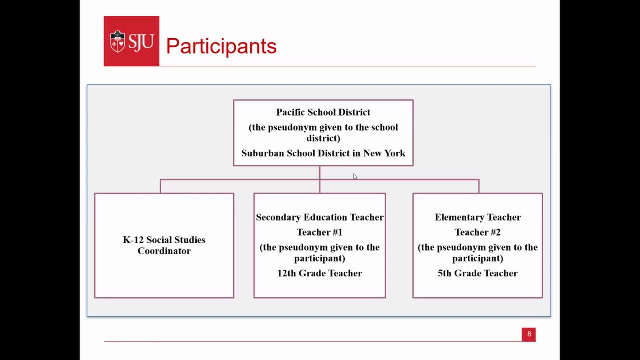 the pseudonym given to the participant, which is a fifth grade teacher who has 28 years of teaching, 22 of them in the Pacific School District, and has spent 19 years in third grade and three years of teaching in the fifth grade. 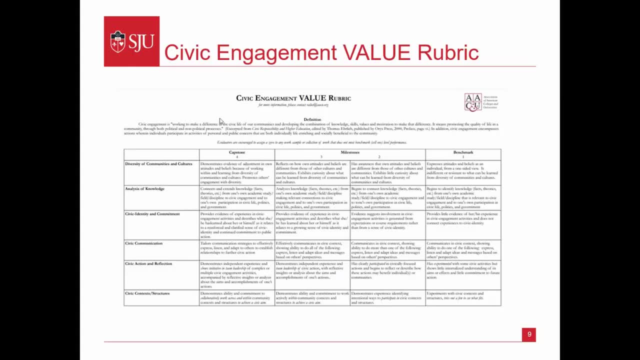 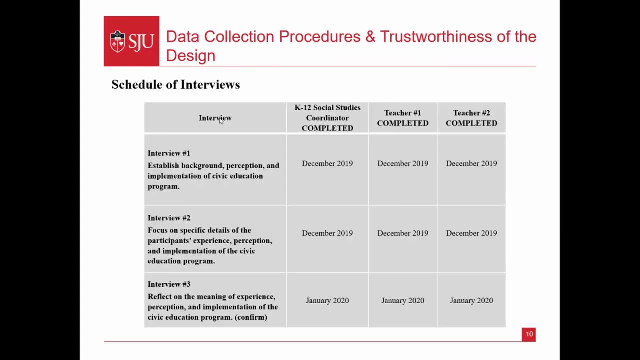 Here is a copy of the study: A specific engagement value rubric that was used in the study as interviews. Document analysis was taking place. In addition, a schedule of interviews when data collection procedures and trustworthiness of design occurred. Interview one, for example, in the K to 12 social studies. 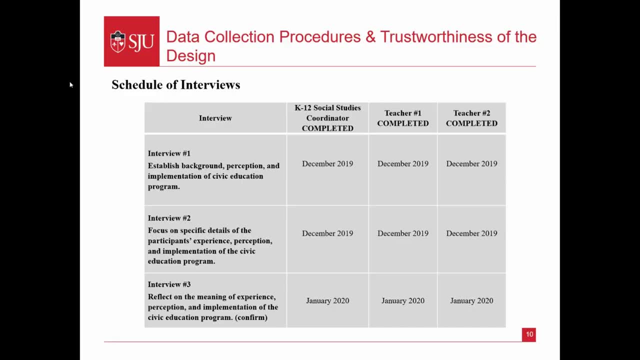 coordinator was completed in 2019.. It established background, perception and implementation of civic education program. The second interview took place in December 2019, the focus on specific details of the participant's experience, perception and implementation of the civic education program. 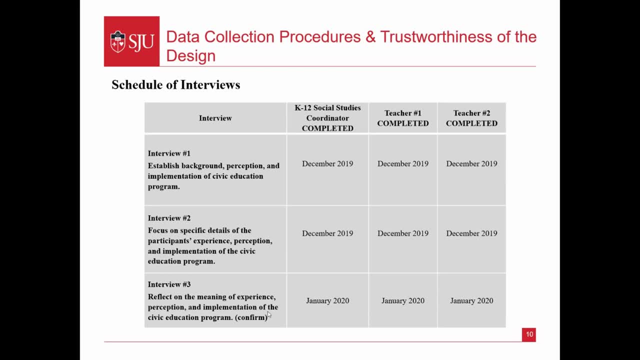 The third interview- January 2020, took place to reflect on the meaning of experience perception- implementation of civic education program. At that time, the data was being confirmed. Likewise, it was similar done to teacher number one and teacher number two. 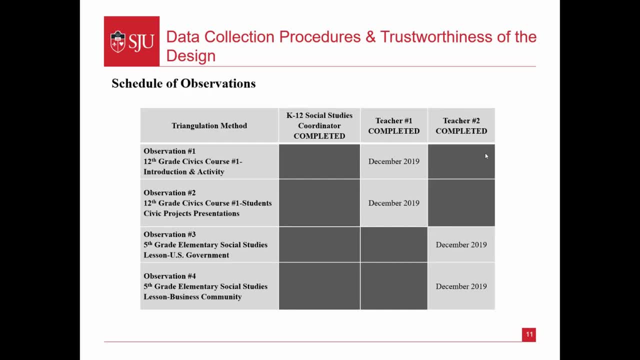 In addition, through myself, I came into classrooms and observed teacher one in December 2019, in 12th grade civics course introduction activity, And the second observation that took place focused on civic student civic projects and presentations for teacher number two, with the elementary level, took place in December 2019.. When went in and observed, 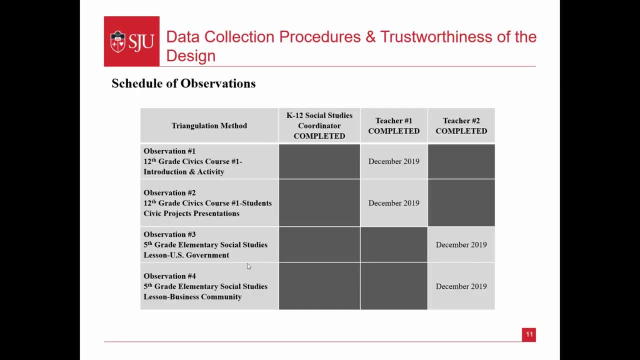 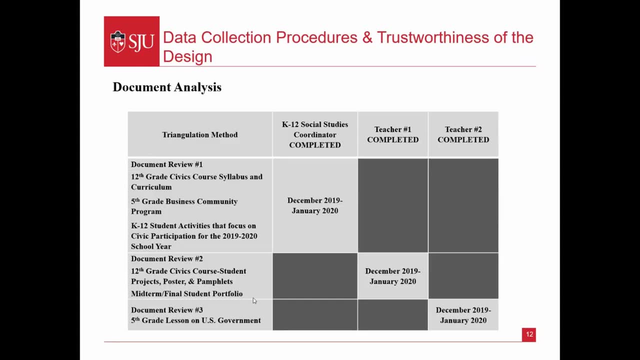 fifth grade elementary social studies lessons in the US government. and then the second Preservation came place in the fifth grade elementary, with focusing on lessons on business and community. for the triangulation method, the document analysis that took place between December 2019 and January. 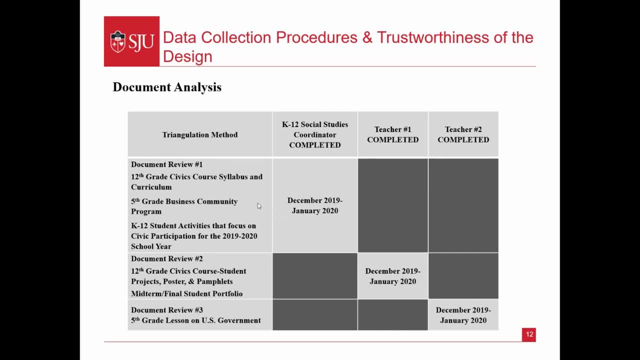 2020 for all three participants. documents that took review with a 12th grade civic course syllabus and curriculum, the fifth grade business community program and the K to 12 student activities that focuses on civic participation for the 2019 and 20 school year. the document review. 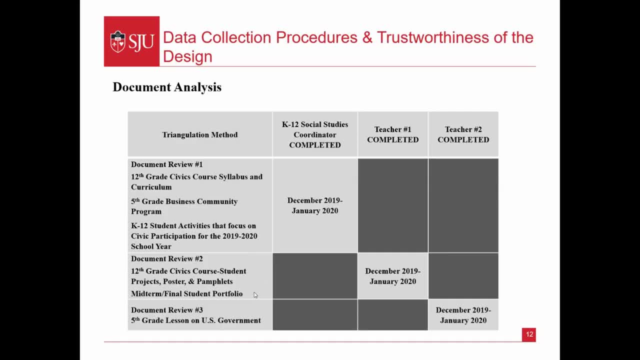 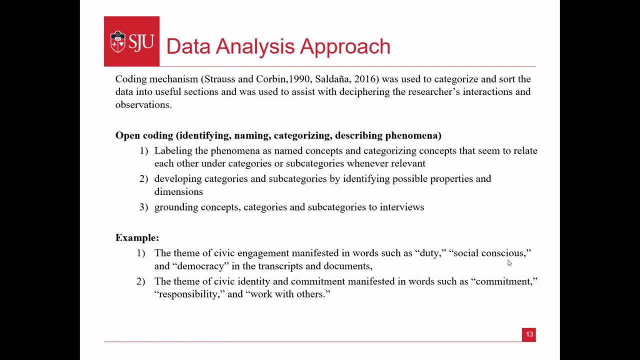 To. it was a 12th grade civics course: student projects, posters and pamphlets, midterm final student portfolio and Document review. number three was fifth grade lesson on US government. The coding mess Mechanism that took place was open coding, which is identifying, naming, categorizing, describing the phenomena by Strauss, Corbin and 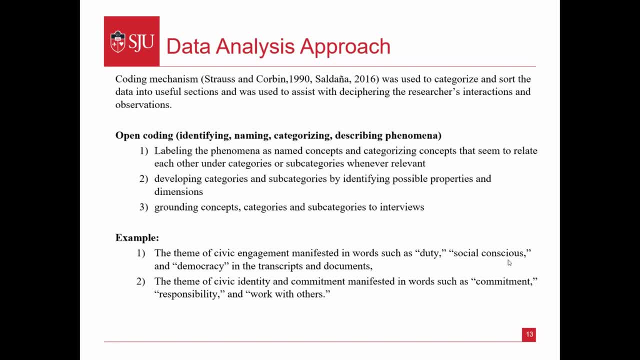 Saldana. it was used to categorize and sort the data into useful sections. It was used to assist with deciphering the research, interaction and observations, for example, The theme of civic engagement Manifest in words such as duty, social conscious and democracy in the transcripts and documents. 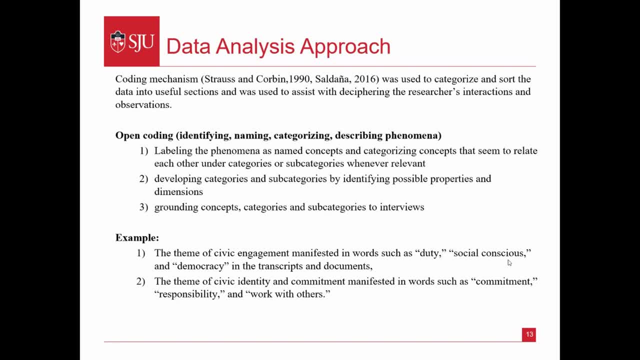 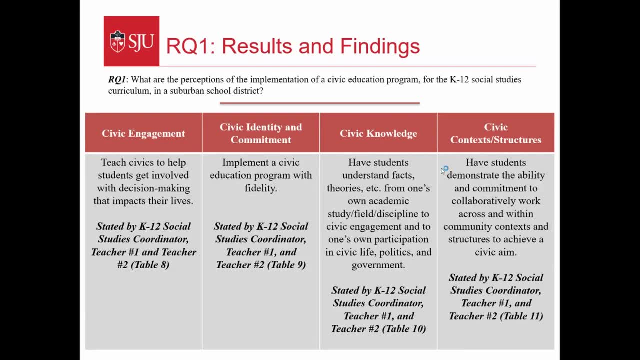 They seem the theme of civic identity and commitment manifest in words as commitment, responsibility and work with others. and Here are some of the findings that took place for research. question one: What are the perceptions of the implementation of civic education program for the K to 12 social studies curriculum and suburban school district? 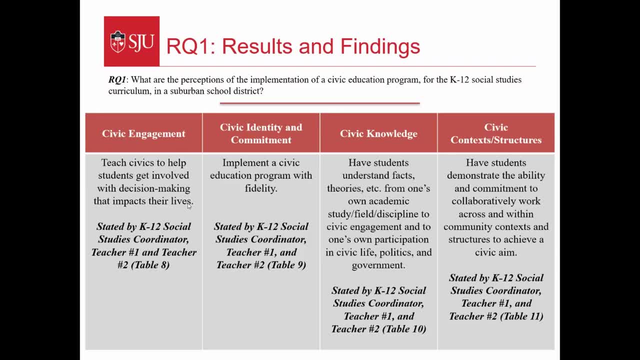 We have themes that came across: civic engagement, Teach civics to help students to get involved with decision making that impacts on their lives. So if you're looking at my dissertation, stated by the K to 12 social studies coordinator and teacher one and teacher two, and that can be found in table eight, the 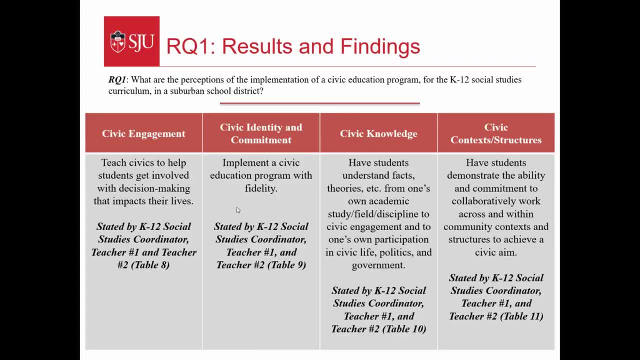 civic identity and commitment to implement civic education education program with fidelity was both- was stated by the coordinator, teacher one and teacher to Civic knowledge. have students understand facts, theories from one's own academic study field discipline to civic engagement and to one's own participation in civic life, politics and government. and 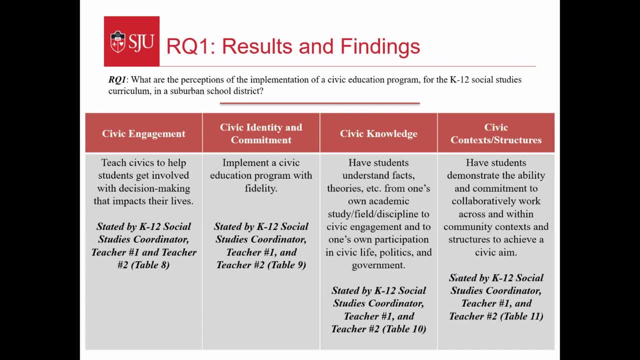 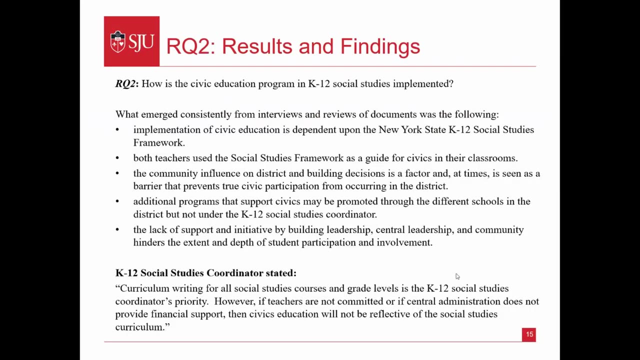 civic context and structures. have students demonstrate the ability and commitment to Collaudally work across within community context and structures to achieve semi-game? and that was stated by K to 12 social studies coordinator teacher one and teacher two and can be found in table eleven For research. question number two: has a civic education program in K to 12 social studies implemented? 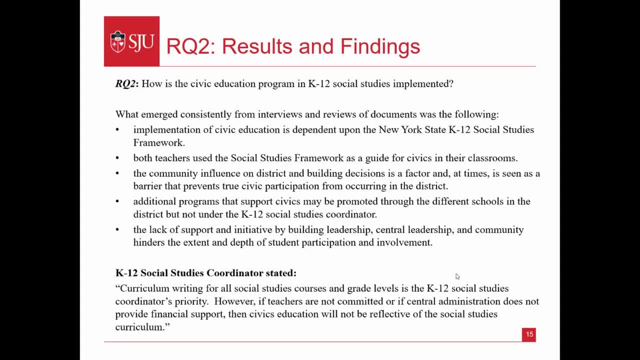 What emerged consistently from these interviews and reviews of documents were the following: the implementation of civic education Dependent upon the New York State framework. both teachers have used the social race framework as a guide for civics in the classroom. the community influence on district and building decision is a factor and in times is seen as a barrier for 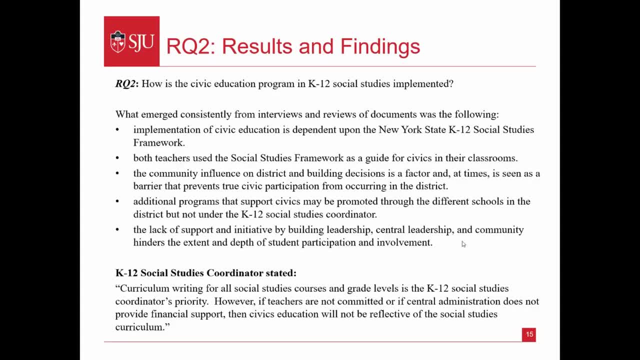 That prevents true civic participation from occurring in the district. Additional programs that support civics may be promoted through the different schools and districts, But not under K to 12. social studies coordinator and the lack of support initiated by building leadership, central leadership and community hinders the extent and depth of student participation and involvement. so 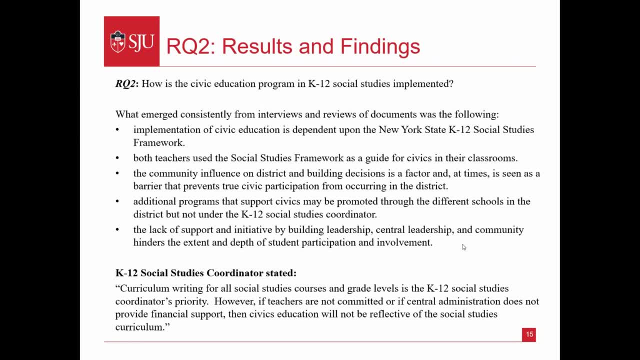 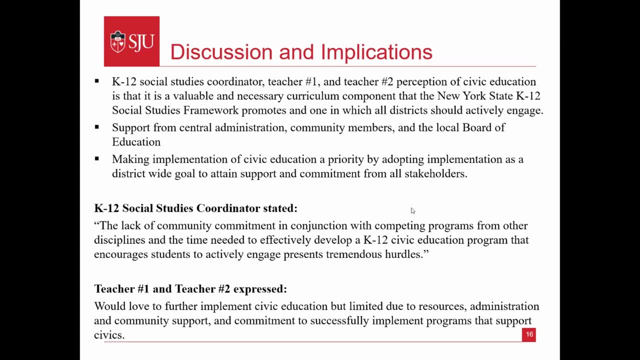 For evidence: K to 12 social studies coordinator. stated curriculum writing for social studies courses and grade levels in K to 12 social days Coordinators is a priority. however, teachers are Not committed or if the central administration does not provide financial support, then civic education will not be reflected of the social studies curriculum. 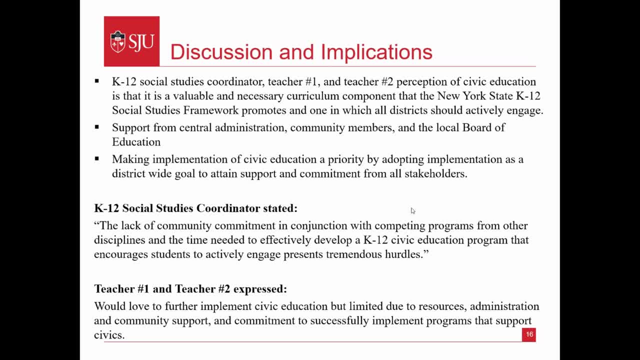 Now for the discussions and implications. Some have stated K to 12 social days, coordinator teacher one and teacher to perception of civic education. is that value and necessary curriculum support from central administration, community members and the Board of Education, and making implementation of civic education a priority by 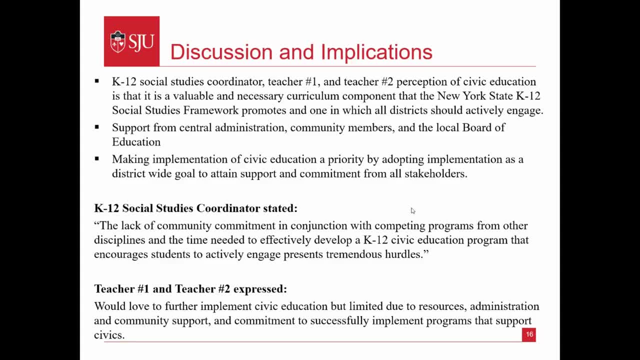 Adopting implementation as a district-wide goal to retain support and commitment for the stakeholders. So, for instance, K to 12 social studies coordinator stated the lack of community commitment in conjunction with competing Programs from other disciplines at the time. need to effectively develop a K to 12 civic education program. encouraged students to actively engage. 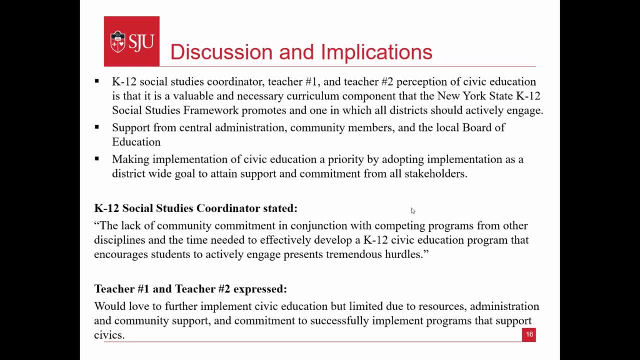 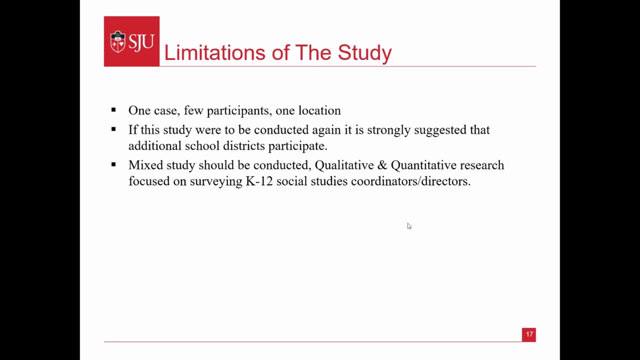 presence, tremendous hurdles, teacher one and teacher to express. would love to further implement civic education, but limited to two resources: administration, community support and commitment to successfully implement programs to support civic education. Here are some limitations of the study: one case, few participation, one location. If the study was to be conducted again, 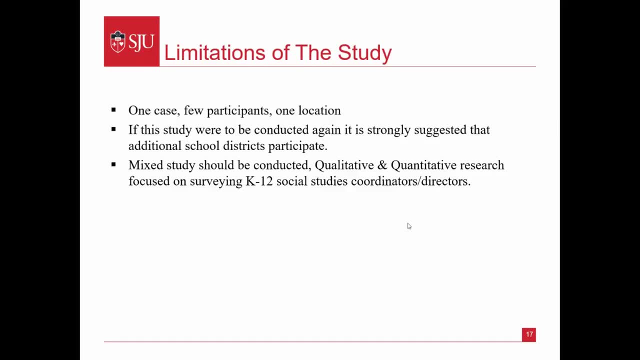 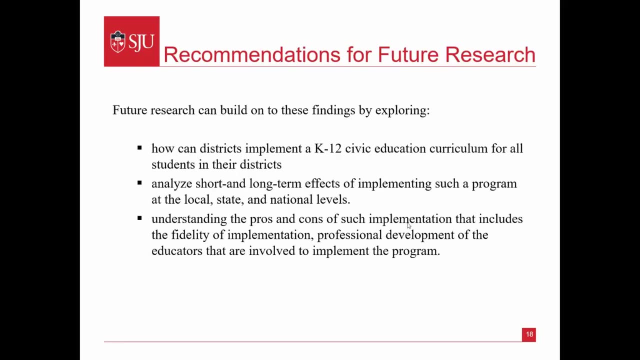 It is strongly suggested that additional school districts participate. a mixed study should be conducted. qualitative and quantitative research focusing on serving K to 12 social studies coordinators and directors. recommendations for future research. how can districts implement on K to 12 civic education curriculum for all students in the district? 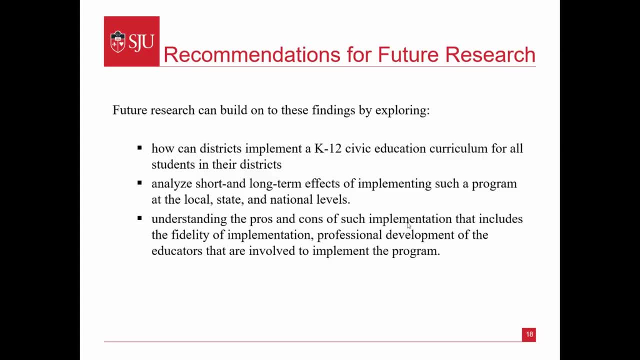 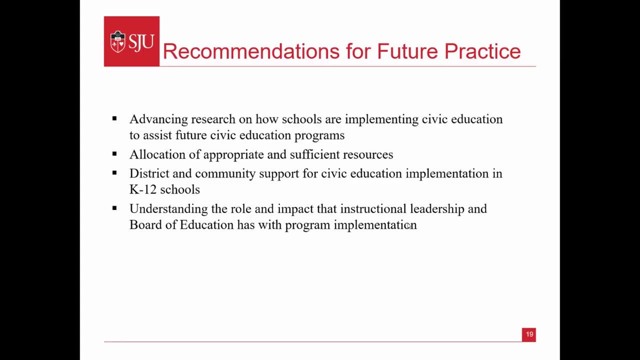 Analyze the short and long-term effects of implementing such a program at the local, state and national level. Understanding the pros and cons of such implementation includes fidelity of implementation, professional development of the educators that evolved to implement the program. in addition, advanced researching and how schools are implementing civic education to assist future civic education programs. 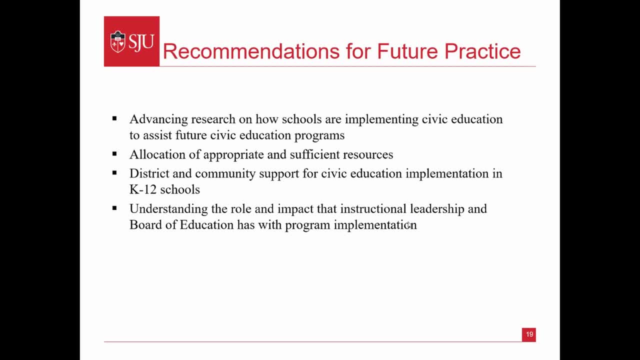 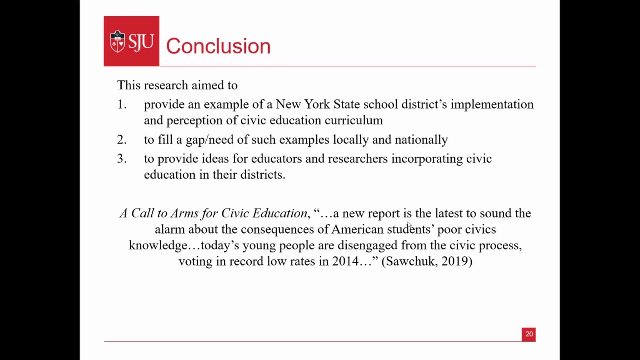 allocation appropriate sufficient resources, district and community support for civic education implementation in K to 2 school, K to 12 schools, and Understanding the role and impact the instructional leadership and Board of Education has within the program implementation. To conclude, the research aimed to provide an example of New York State School District implementation perception of civic education curriculum. 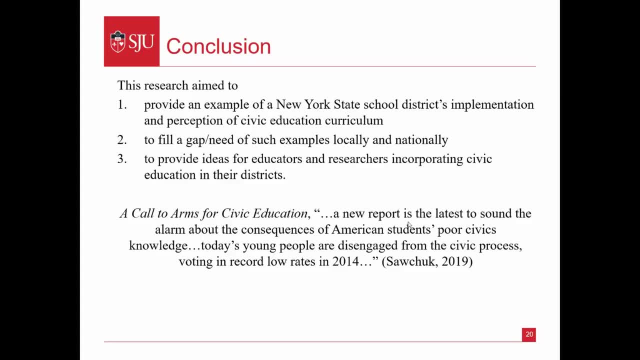 Try to provide a fill to fill a gap or a need of such examples locally and nationally. provide ideas for educators and researchers incorporating civic education in the districts. A call to arms for civic education. I wanted to end off with a quote. a new report is the latest to sound alarm about the consequence of American students. 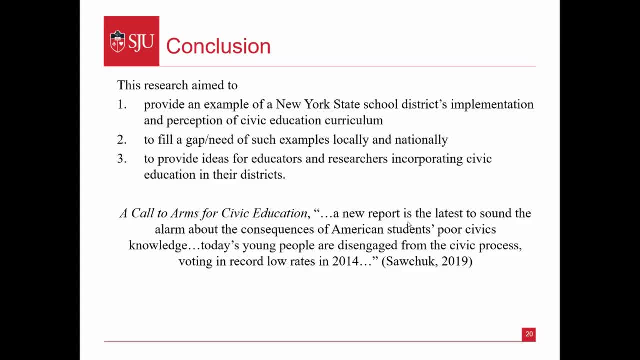 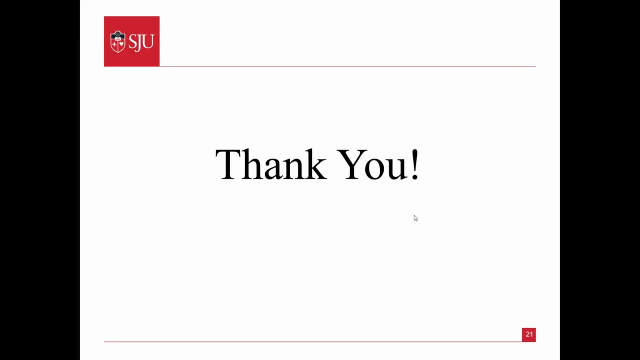 Poor civics knowledge. today, young people are disengaged from civic process voting and record low rates in 2014. If you have any questions concerns, please always reach out for me and thank you for your attention. You.